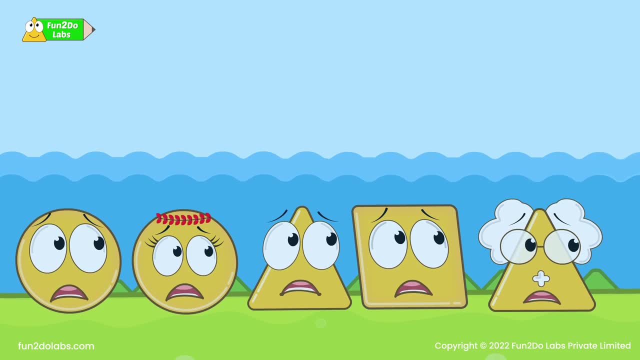 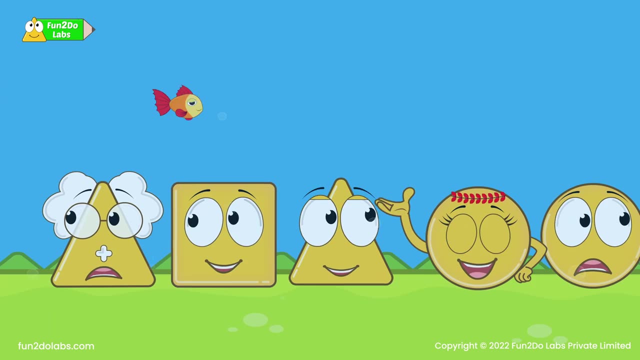 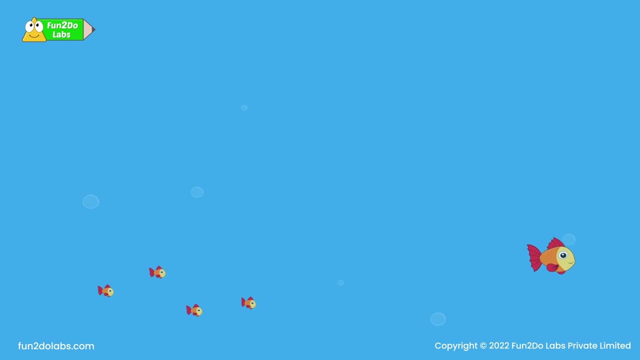 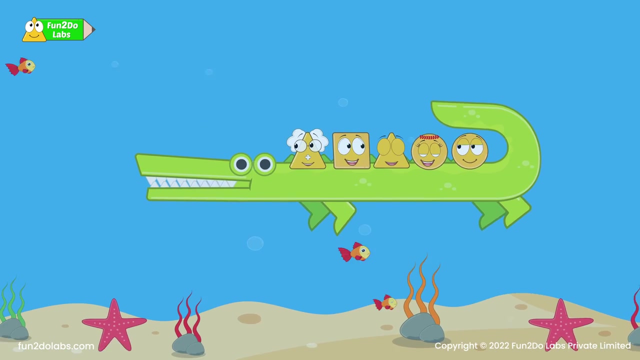 Everybody is even more scared and nervous now. Max swiftly dives underwater, carrying everyone. Wow, The underwater world is equally colourful. There are many types of big and small fish. The underwater plants look so different and yet pretty. The kids are astonished to see the beauty of the underwater world. 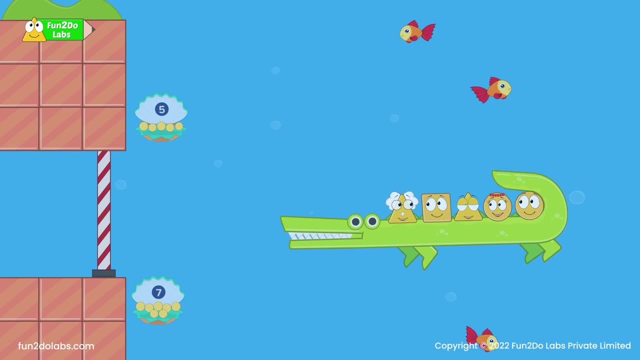 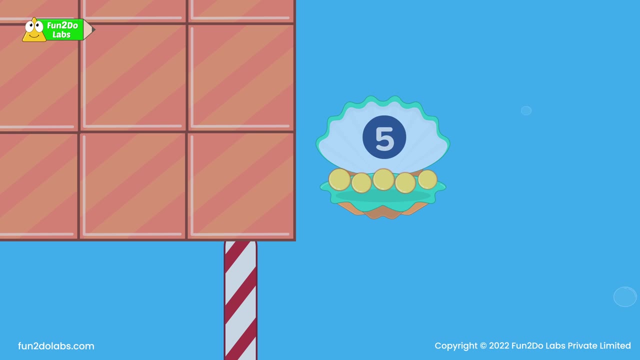 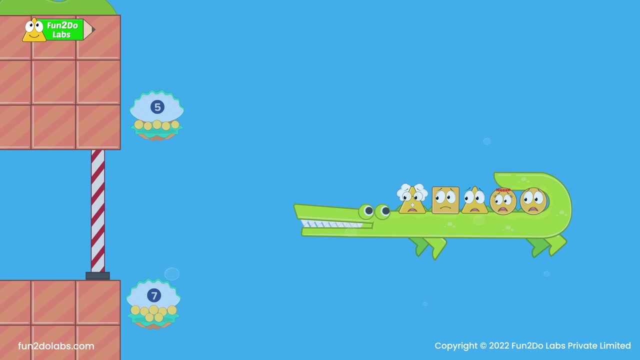 Soon the first door arrives, Max stands near the door Time to feed me. Which number should I eat? There are two shells: One on the top with five pearls and another one in bottom with seven pearls. Which shell shall I eat? 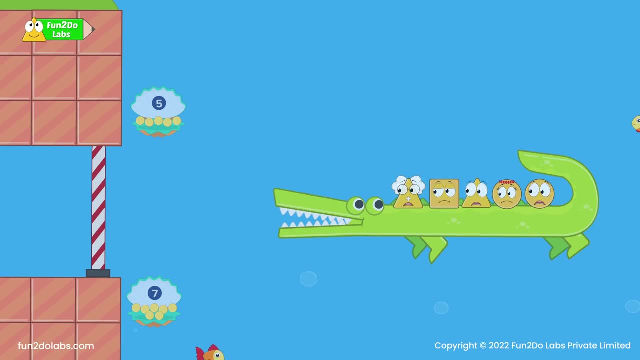 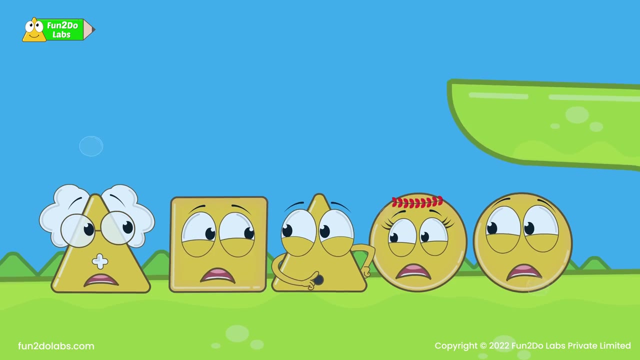 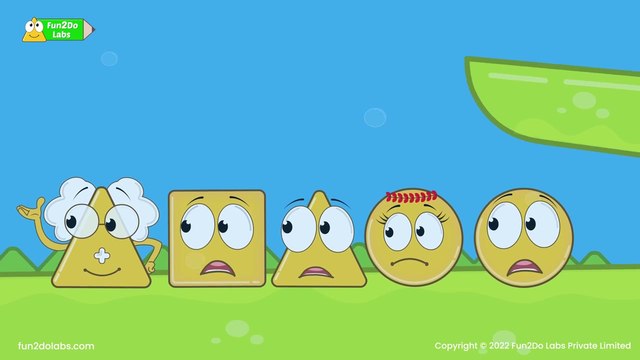 Eat the shell with five pearls. I will give you one last chance, Otherwise be ready to stay here forever. Treeho asks Squirrel to keep quiet and stay calm. Children look inside the number shells carefully. The shell with the number seven has seven pearls. 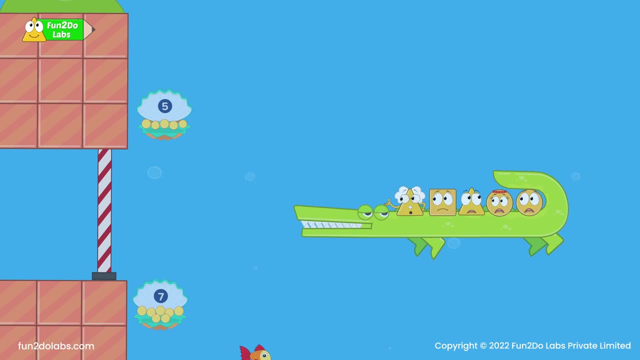 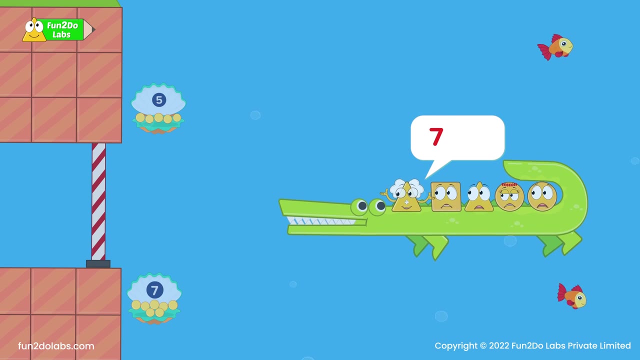 and the shell with the number five has five pearls. Which shell has more pearls? The number seven shell. Yes, correct, So number seven is greater than number five. They order Max to eat the number seven shell and the door opens. Max is happy and the kids are relieved. 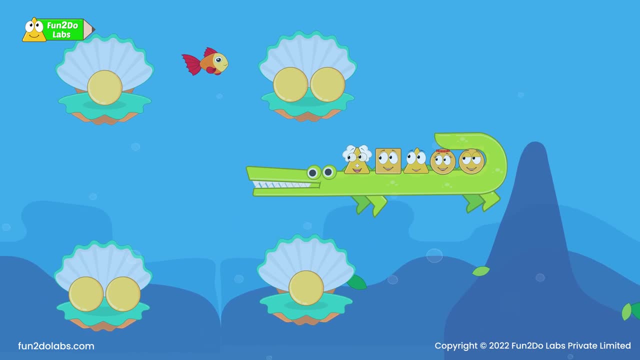 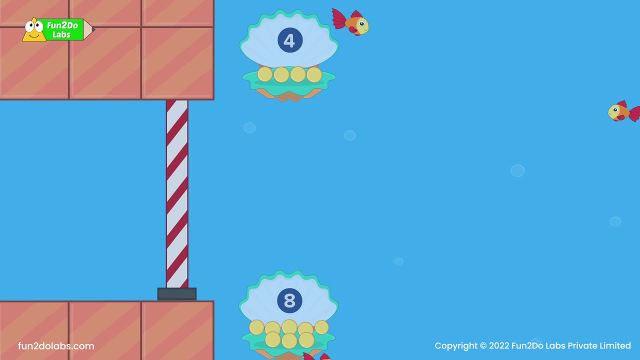 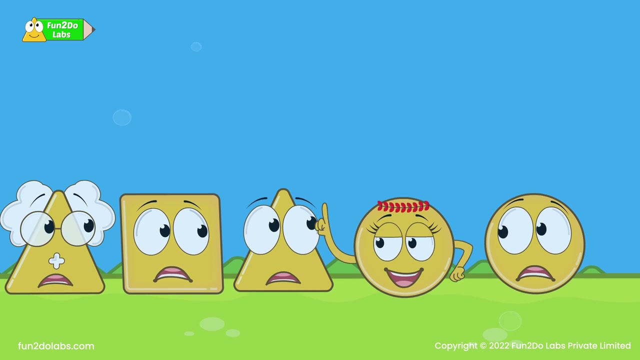 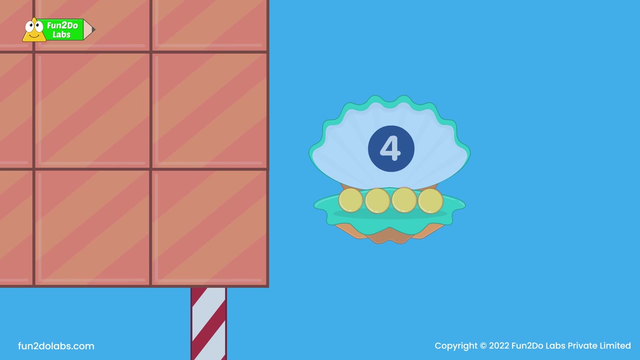 Behind the door there are so many shells with beautiful shining pearls, Soon the next door arrives. This time the door has two shells with numbers four and eight. There are four pearls in one shell And eight pearls in the other shell. The shell with eight pearls has more pearls than the other shell. 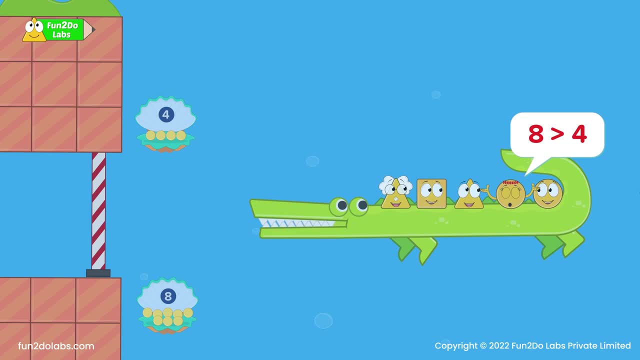 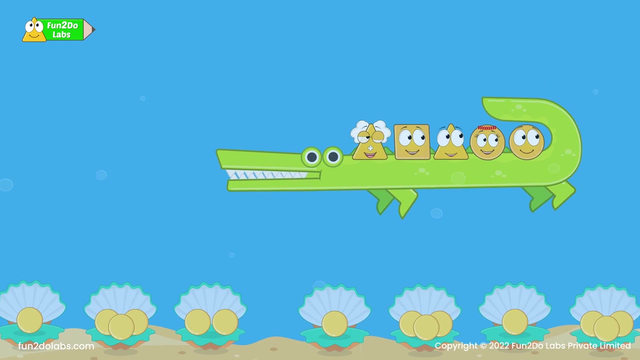 This means number eight is greater than number four And number four is less than number eight. Eat the shell with eight pearls, Max. The door opens immediately. This time, the door takes them to another beautiful side of the underwater world for the kids.